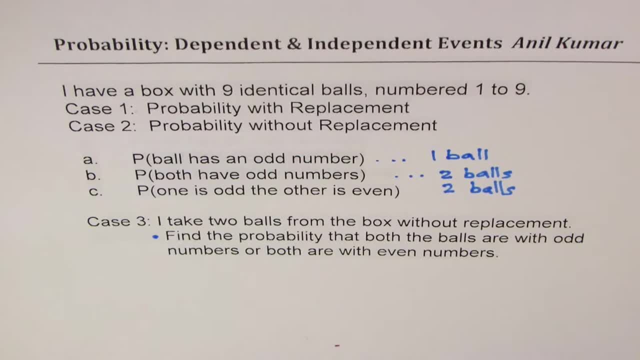 odd numbers or both are with even numbers. So this is a great example. It actually covers a lot of concepts. So let me just show you what we are working on here. So let me just show you. This is a very simple display of what the three balls we are working with. We have a box here and in this box we have different balls. 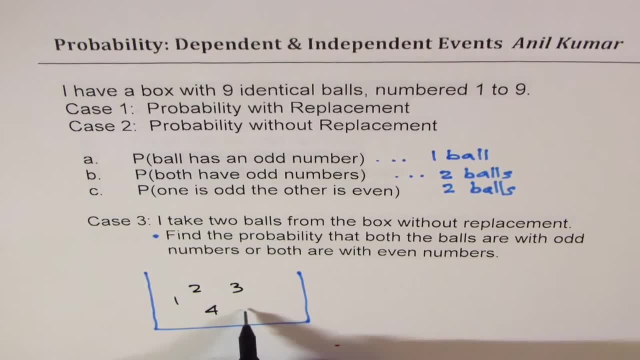 So let's say this, number them as one, two, three, four, five, six, seven, eight, and let's say nine. As you can see, let me circle the ones which are odd, since most of the time we are interested in odd One, three, five, seven and nine. 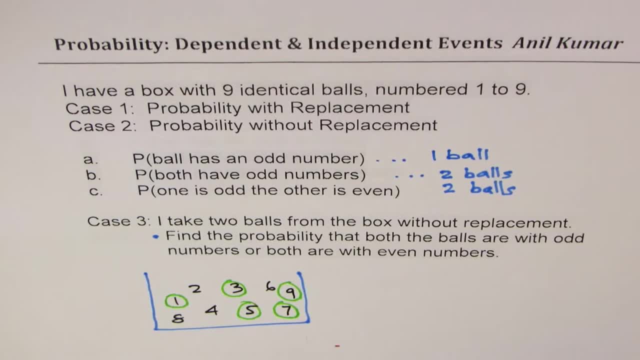 So we have 1,, 2,, 3,, 4, 5 odd balls, correct? So in the first case, when we are saying what is the probability that when I pick up a ball from this group it is an odd number? 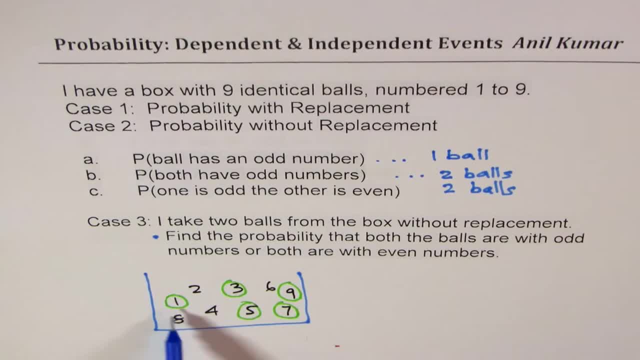 So in case of a probability, success is what is the possibility of getting an odd number? So the probability for getting odd ball is number of success over number of total. Actually, I should not have used the word S, because S is used for sample space. 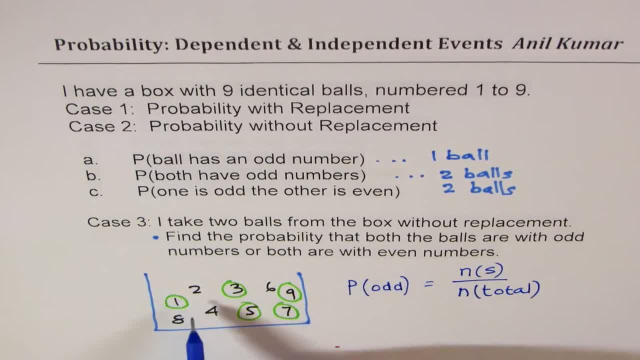 Let me write total here, right, Okay Now, in this case the odd balls are 1,, 2,, 3,, 4,, 5.. And therefore I get 5 over. total number is 9.. So that becomes the answer for part A. 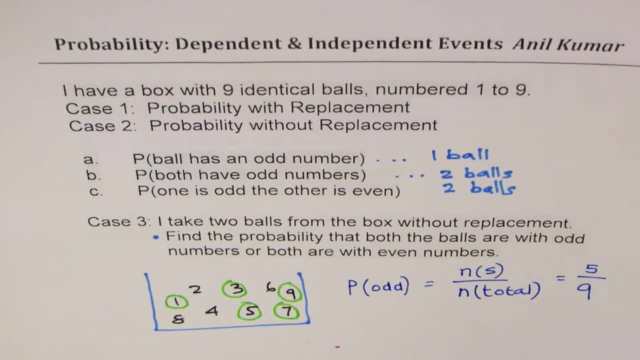 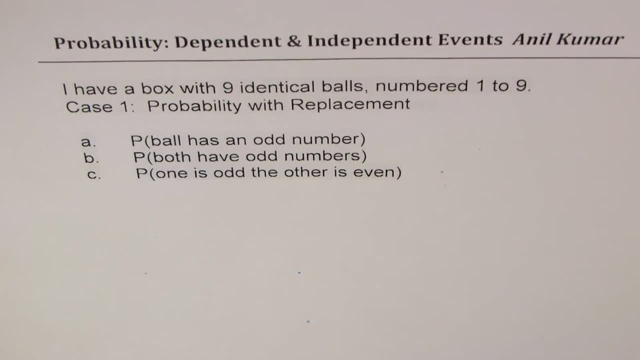 Now let us discuss part B and C, with reference to both the cases, when we are talking about replacement or without replacement. So again, I have a box with 9 identical balls, number 1 to 9, case 1, probability with replacement right. 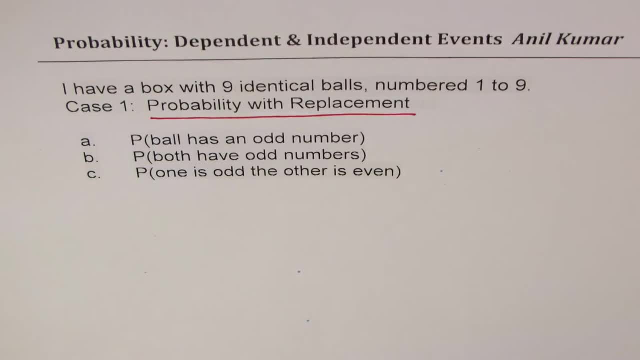 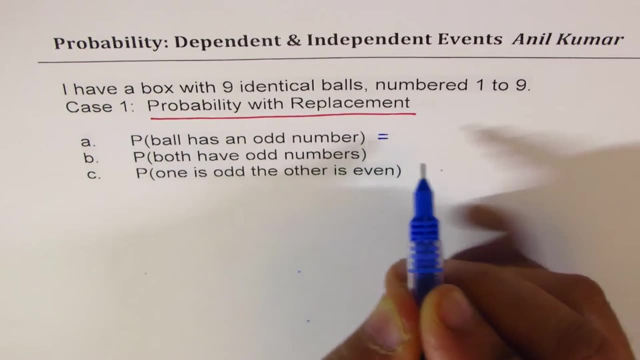 So we are talking now about probability with replacement, So I will not do the first part. we already have seen In case of 1 ball. the probability in this case is equal to 5 over 9,. right Now let us look into the other two cases. 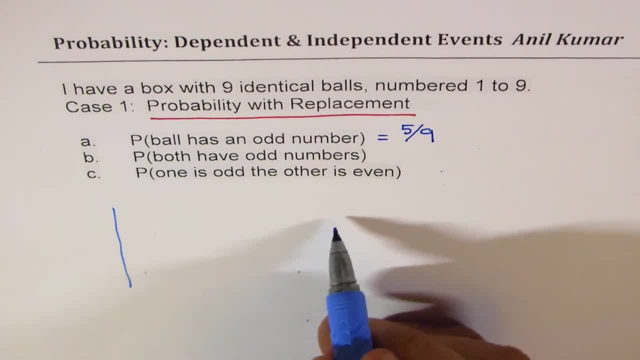 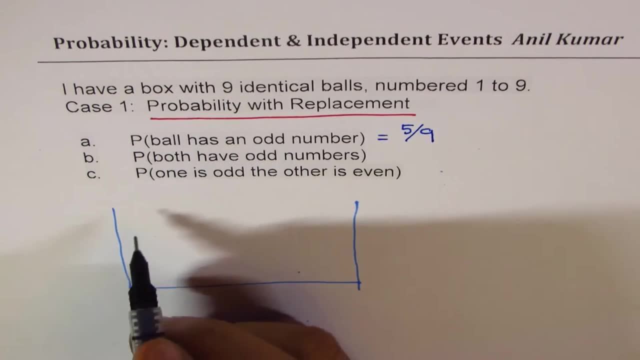 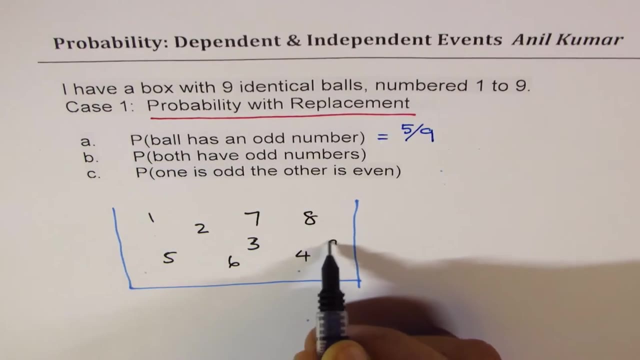 So again, let us look into this box. Let me make a bigger box this time. So we have the numbers, which are 1,, 2,, 3,, 4,, 5,, 6,, 7,, 8, and 9.. 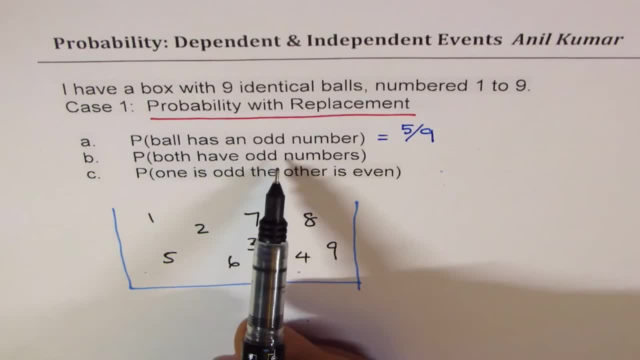 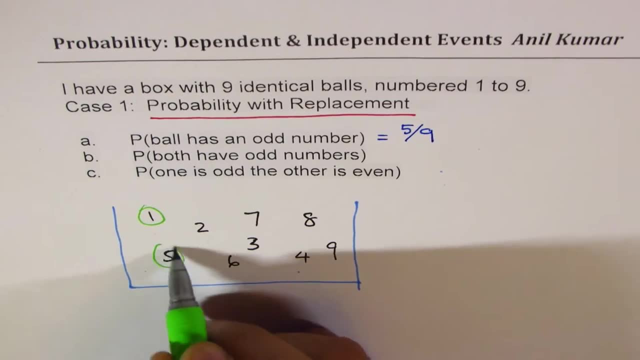 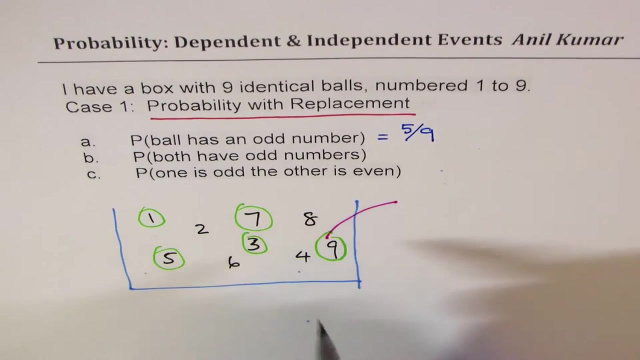 We are looking for picking up both half-odd numbers and with replacement, right? So odd numbers are 1,, 5,, 3,, 7, and 9.. So replacement really means that let us say, if I pick up one of these numbers, what is the probability of picking an odd number. 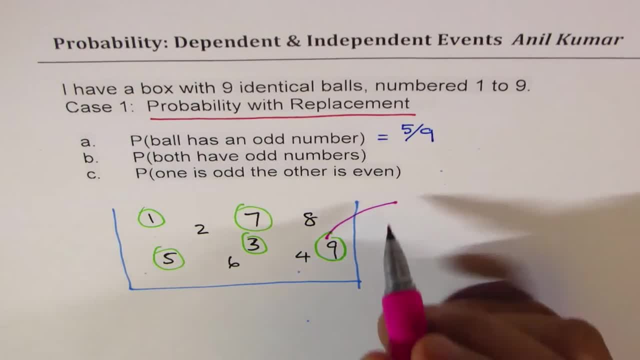 For the first time when you pick it up, it is 5 over 9.. Now replacement means that this ball has been put back. Now you picked it up, but then you replace it. So again, the total number of balls remain same. 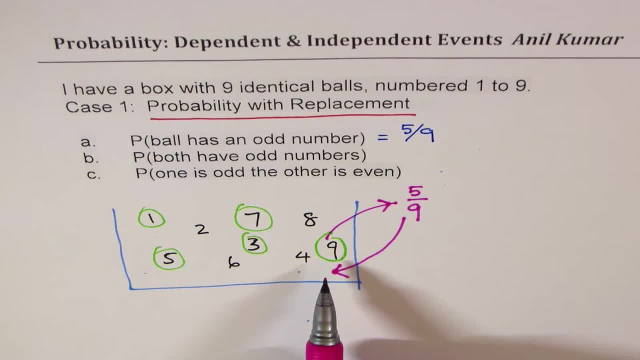 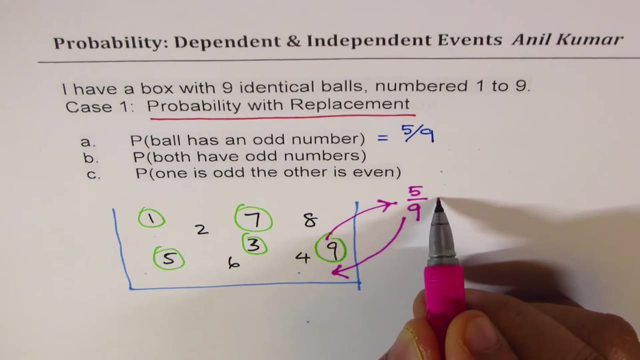 That is, there are total 9 different balls. Different numbers, I mean exactly identical Otherwise. so now I said both odd balls. So second time again, if I pick, I have the same probability right, Because exactly similar situation and we get the same probability. 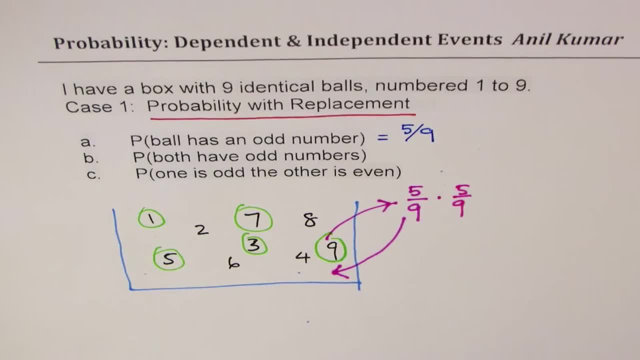 So it is 5 over 9 once again. So what? we also say that this event is independent of the first. I mean the second event is independent of what happened before it, correct, Since it does not change the scenario. So that is our take on independent. 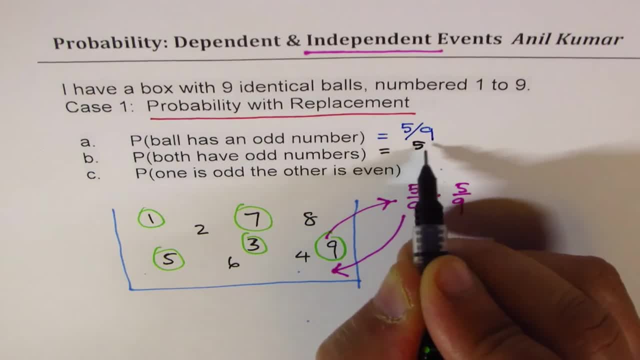 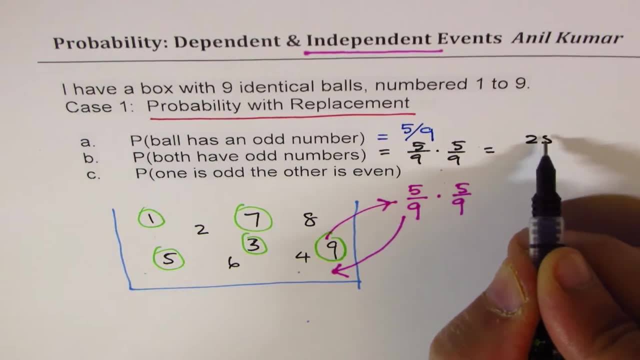 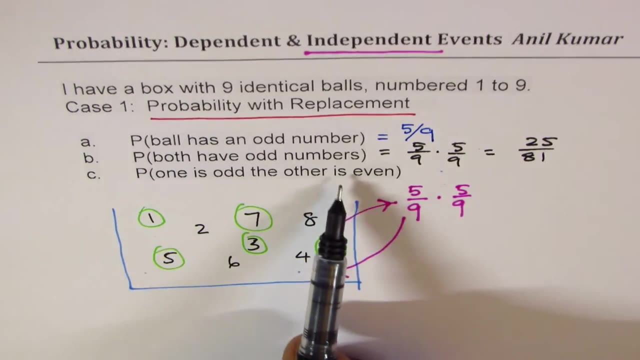 So both half-odd numbers will be 5 over 9.. 9 times 5 over 9,, correct. So that becomes your answer, which is 25 over 81.. Now the second case here is: one is odd, the other is even. 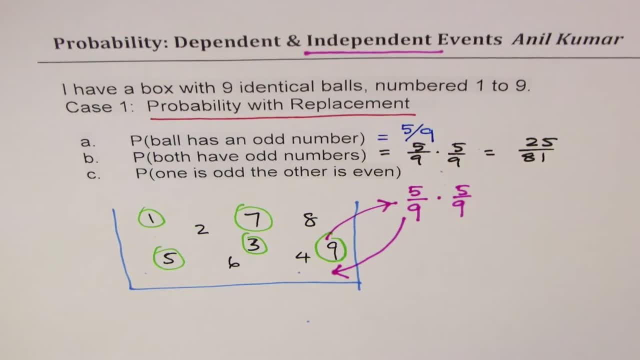 Now for the second case. if one is odd and the other one is even, then the probability of picking up odd is 5 over 9.. Now we are talking again with replacement, So it has been replaced And the other one which you pick up is even. 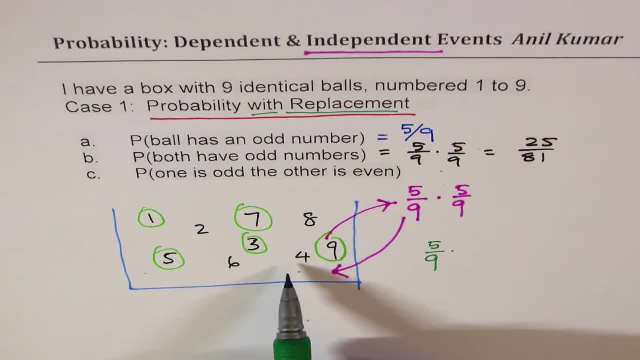 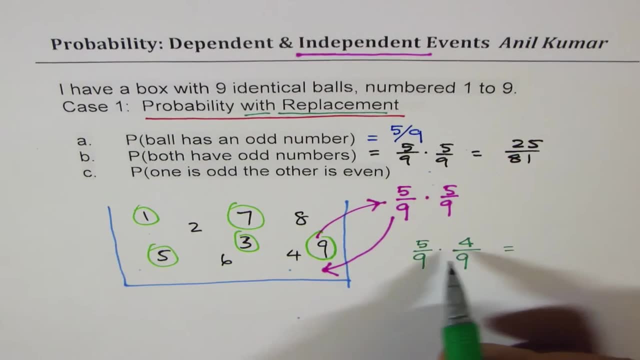 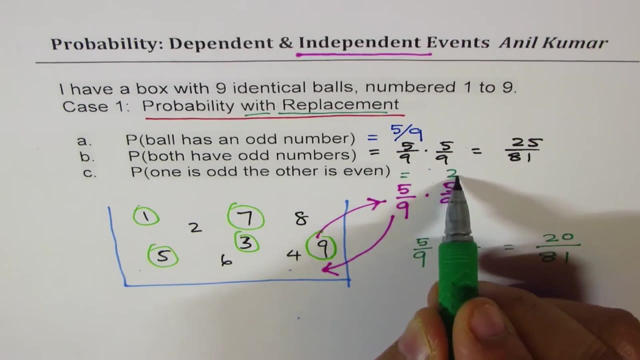 That means the other one could be 4, one of these 4, right, So it is 4 over 9.. What we get here is 4 times 5 is 20 divided by 81. So this probability is 20 over 81.. 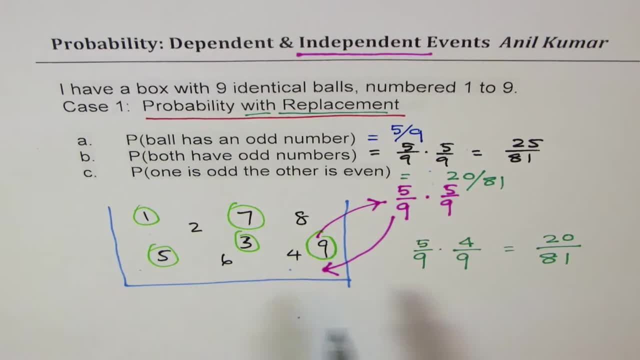 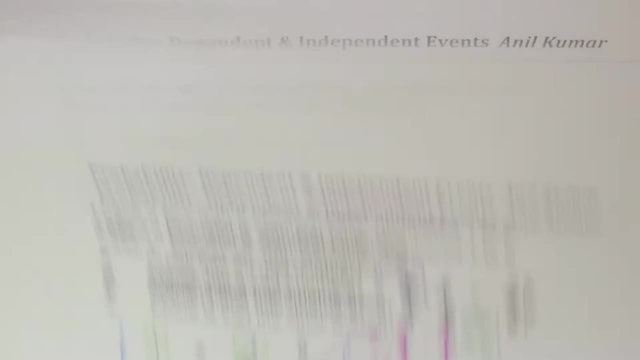 Now, in this particular case, we have mentioned probability using straight formulas. Now we can also make tree diagram to get similar results. So in the next example I will try to draw a tree diagram and then explain you the result. So let's take case 2.. 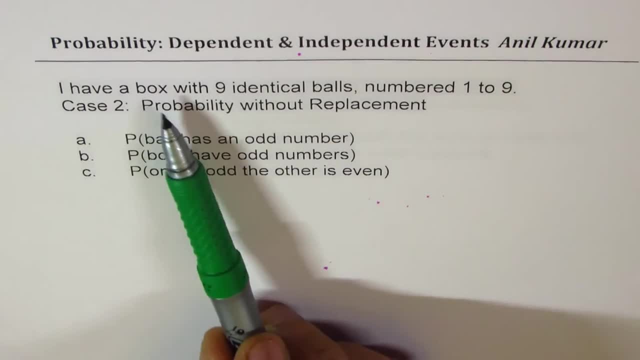 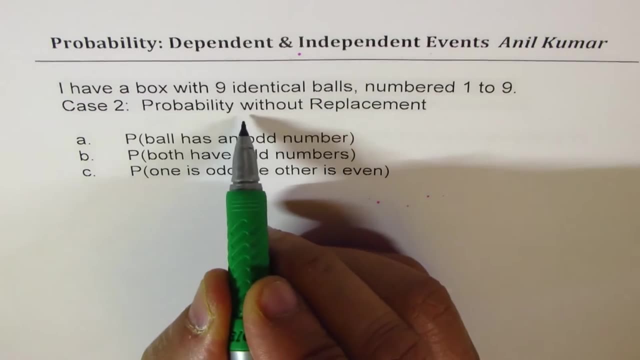 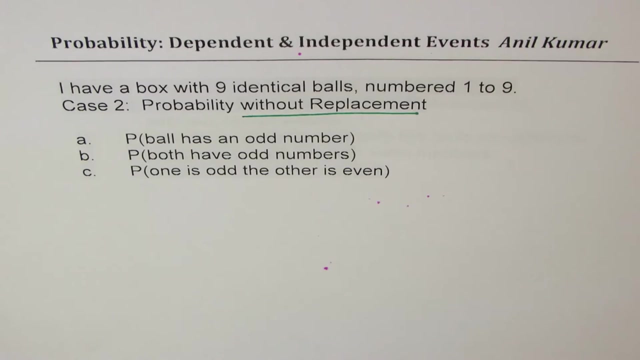 Again, the same question is there for us. I have a box with 9 identical balls, numbered 1 to 9.. We are talking about case 2, which is without replacement, right, Without replacement. So well, in case 1,, as we know, a ball has an odd number. 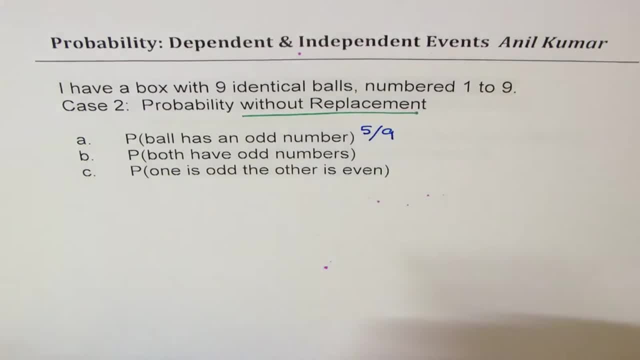 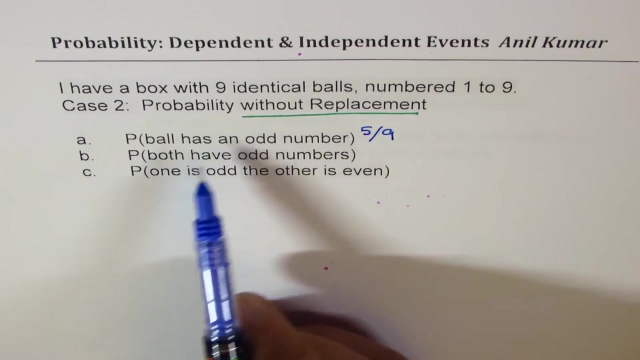 Probability is 5 out of 9.. That is fixed Now. B and C. we'll now look into these cases when both have odd numbers and the other one one is odd, the other one is even. This time I'll answer this question using tree diagram. 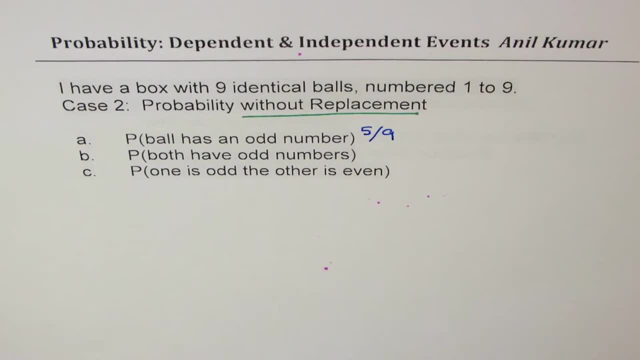 So we are having a different approach, So we'll take tree diagram now. So let us say we pick up one of these balls from 9 identical numbered, 1 to 9. In that case we could get either odd number or an even number, right? 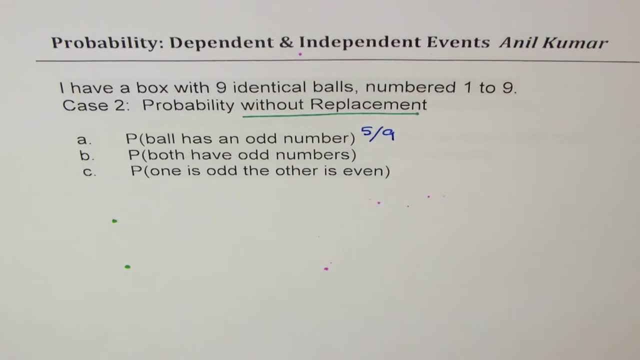 So that is the possibility. We could get either odd or even So. so when you do this operation, it could be odd number or even number. Probability of getting odd number is 5 out of 9.. So we are calling this as odd. 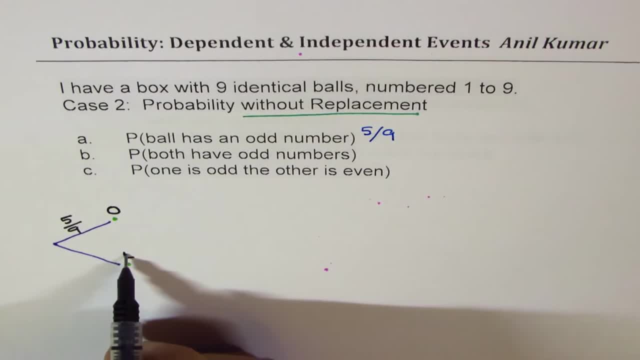 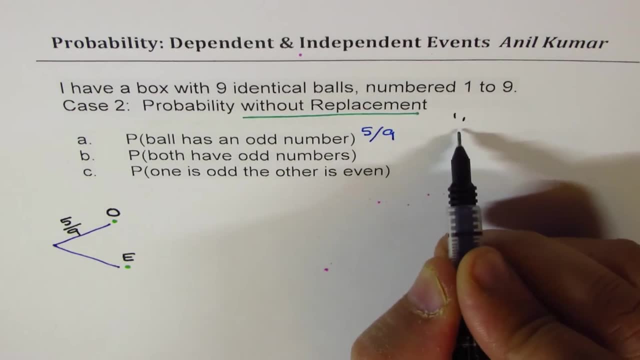 Let me write this as O and even as E. So that is our first pick. The second one, even since the numbers are 1, 2,, 3,, 4,, 5,, 6,, 7,, 8,, 9,, 10,, 11,, 12,, 13,, 14,, 15,, 16,, 17,, 18,, 19,, 20,, 21,, 22,, 23,, 24,, 25,, 26,, 27,, 28,, 29,, 30.. 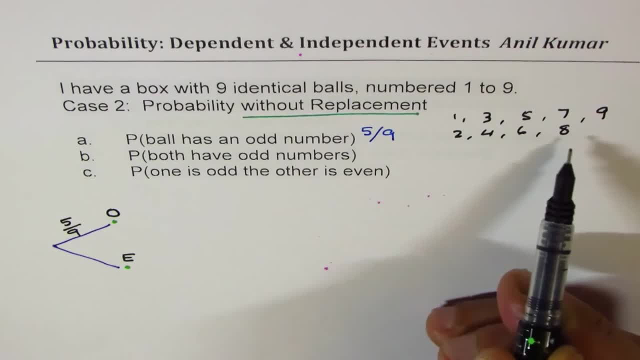 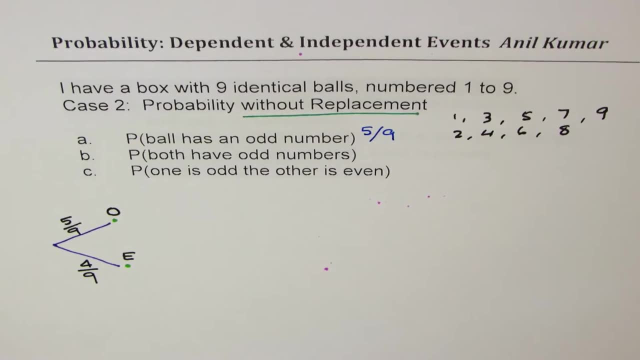 Clearly you can see there are five odd numbers, four even numbers. So for even number, the probability is 4 over 9,. right Now we have to pick the second ball, and that too, without replacement, remember, right? So let's see how to move further from here. 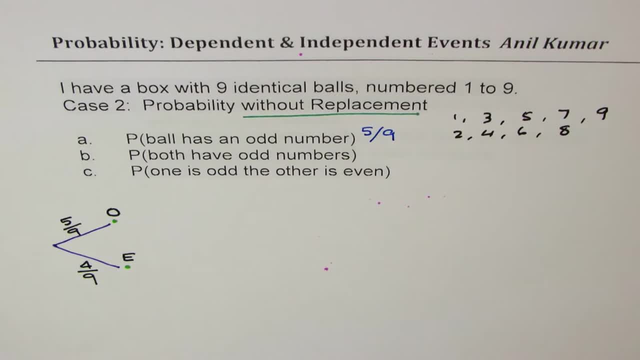 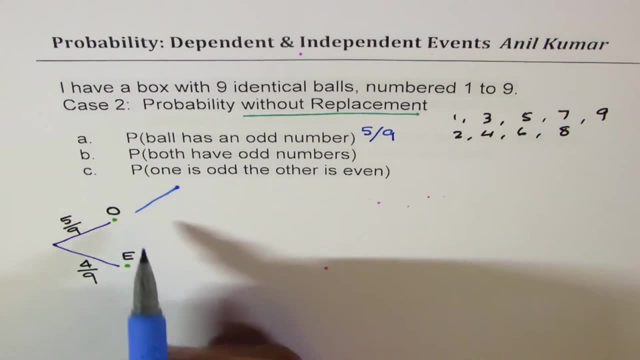 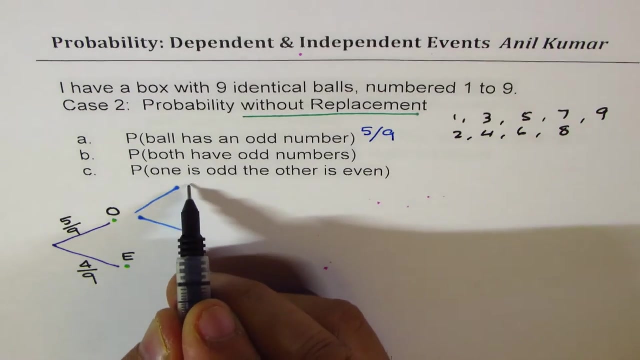 So we are picking up now the second ball. Let us say that in the first case we have drawn odd ball right. so we have two scenarios here in the second row we can get either odd or we can get even. so there are two possibilities: we get odd or we get even right. what is the probability? 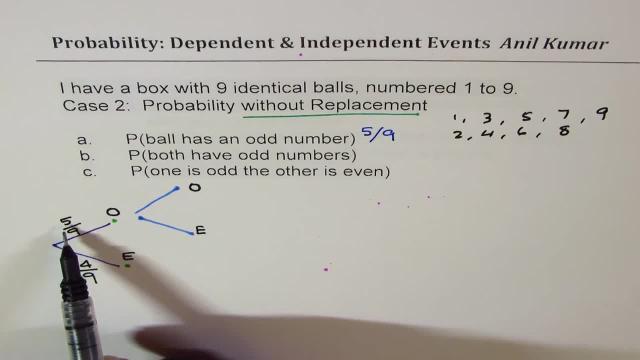 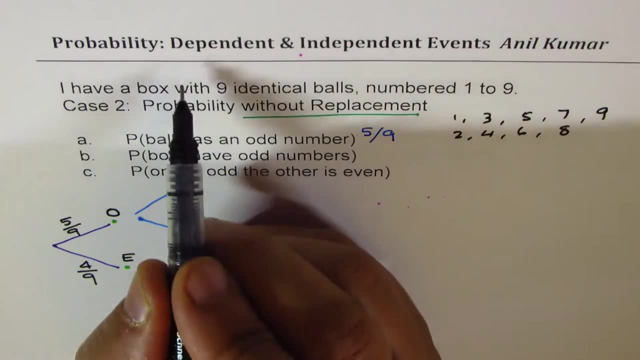 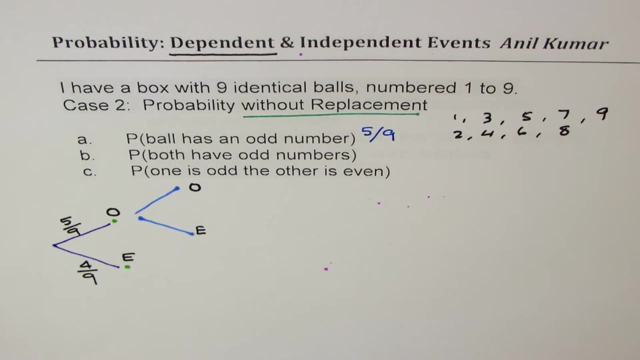 of picking odd. since we have already taken out one odd ball, we have reduced that number to four. you can see, this is a dependent event. perfect. since the scenario has changed, the sample space has changed. we are not left with nine balls, we are now working just with eight. so the denominator 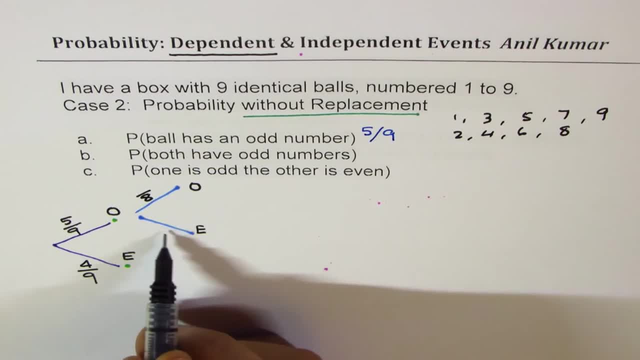 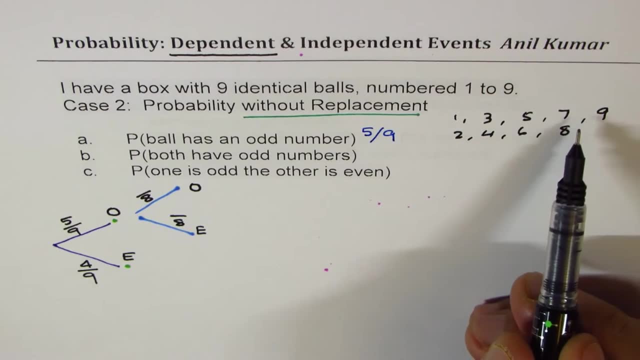 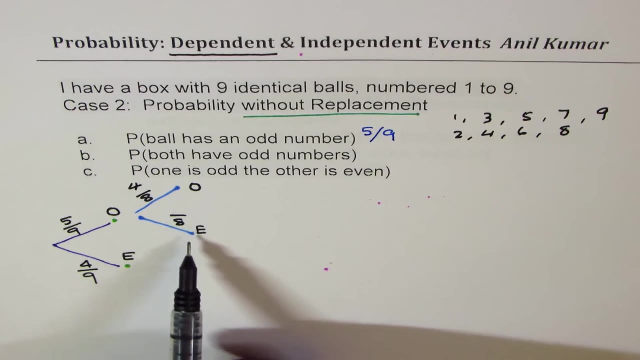 in this case, is going to be eight for both the scenarios. right, it has to be eight. but you picked up odd ball, so number of odd balls reduced from five to four, so this ratio becomes four over eight. on the other hand, number of even balls remain same as four, so it remained four. 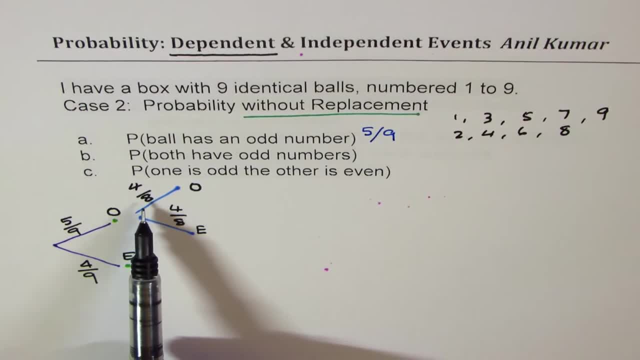 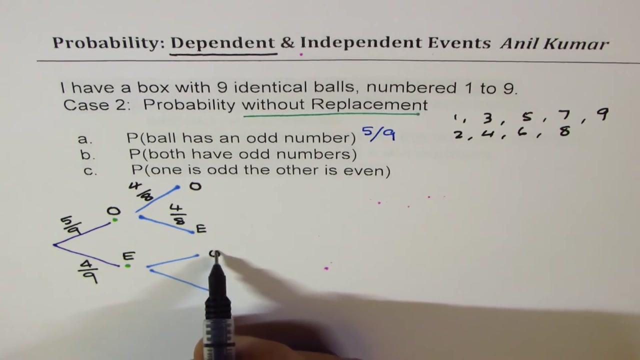 over eight. do you see that? so the sample space change: reduction by one ball, as it was drawn earlier and not replaced, perfect. let's look into the next scenario, which is, if we had taken away even ball, then what right? then what? so in that case also possibility is either get odd ball or even right. so these are the two possible cases. 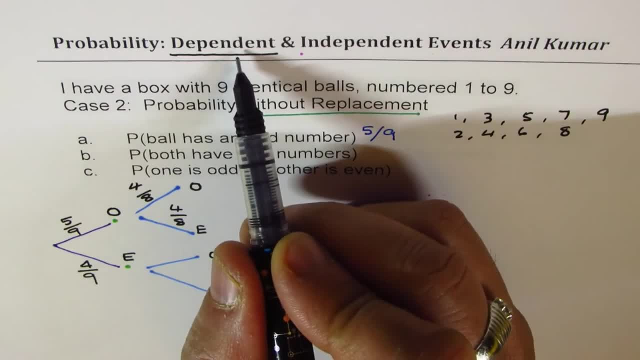 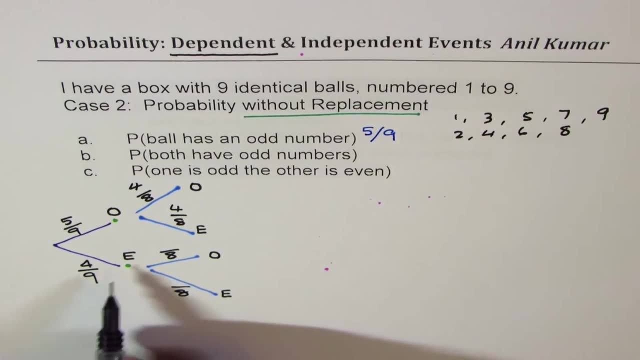 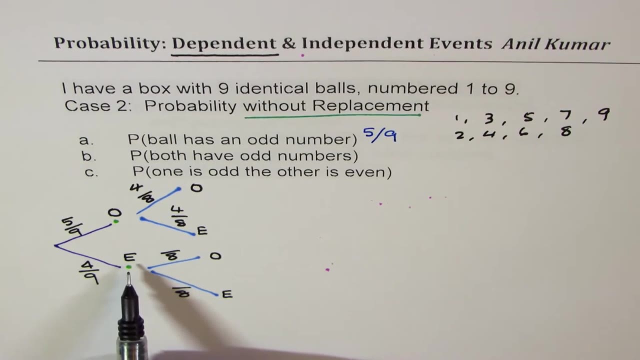 the scenario has changed. it is dependent event, perfect. so there are total reduced number of balls to pick from. it is eight now. one has been already selected randomly, right. in this case, we had actually taken away one even ball. therefore, the number of odd balls are still the same, right. 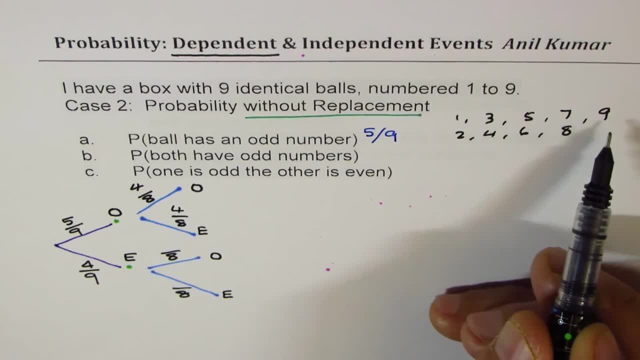 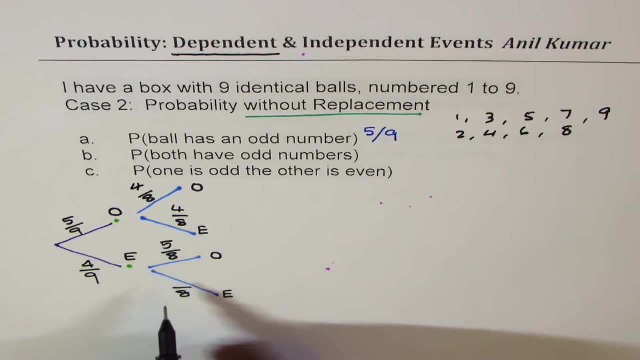 so number of odd balls are one, two, three, four and five. so we get five out of eight, one less than the four even balls, so it is three, right. so we get three out of eight, as the probability of picking up an even ball when already even has been taken out. so this is the 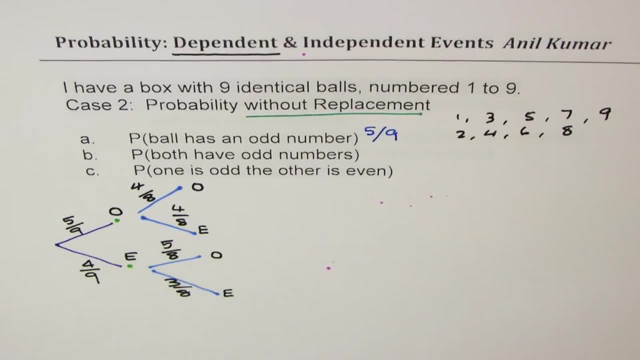 case of without replacement, right? so you see how, when we do without replacement, the numbers are dependent on the previous event. okay, so these are the scenarios for us. let us see what outputs do we get for each. so when we say one followed by the other, then their. 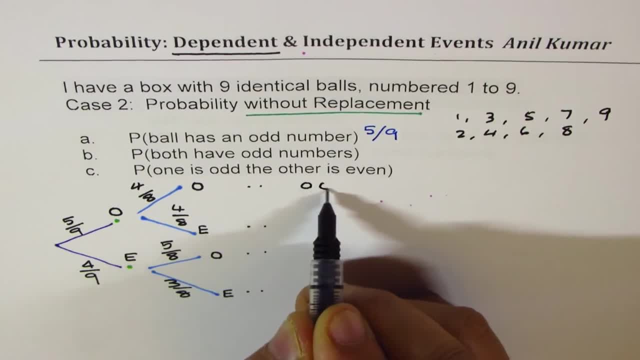 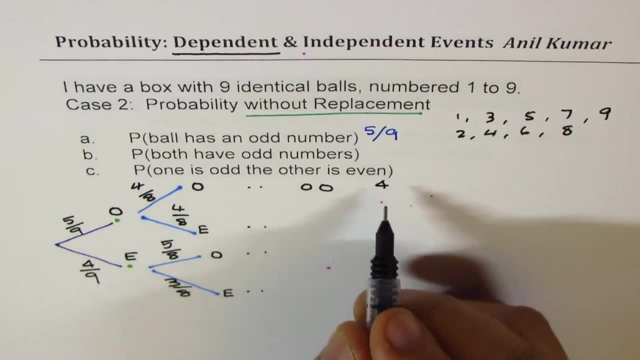 probabilities get multiplied. so for both odd. so let's say we have both odd. in that case it is five times. let me write this as five. i mean, okay, i wrote four over eight. let me write four over eight and 5 over 9. that becomes the product. In this case it is odd and even, and the probability will. 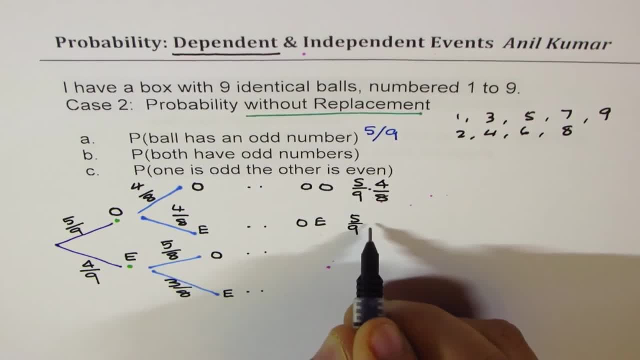 be product of these two, which is 5 over 9 times 4 over 8.. I could have written half also, but purposely I am not doing it. It helps to add at the end: Now: to get even and odd, the probability is 4 over 9 times 5 over 8, and for getting even and even, it is 4 over 9. 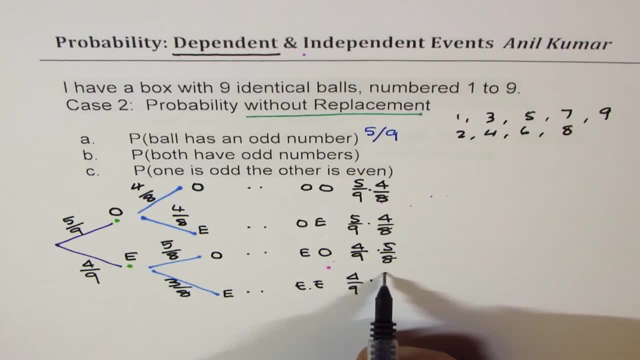 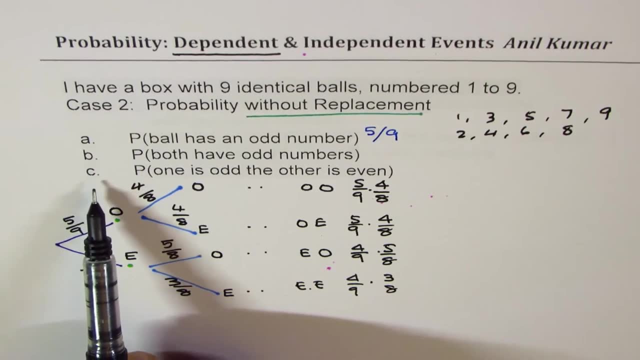 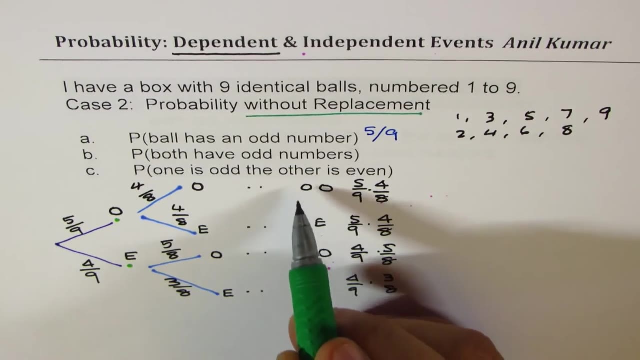 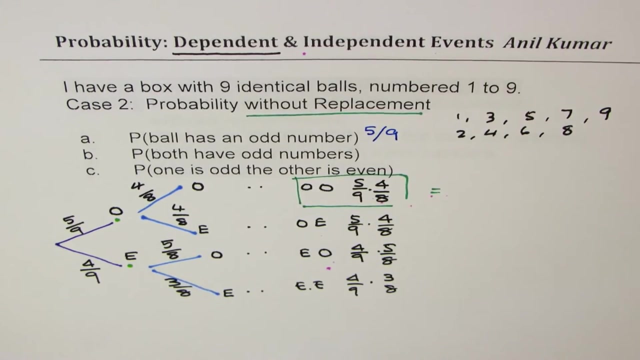 times 3 over 8.. So these are different scenarios. Now we can actually answer part b and c. Part b is both have odd numbers, So both have odd numbers. that means we are looking into the first scenario. Both have odd numbers, right. So we can calculate this number and write that as an answer, right? 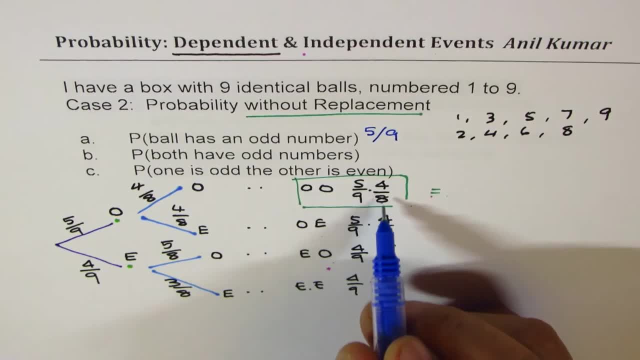 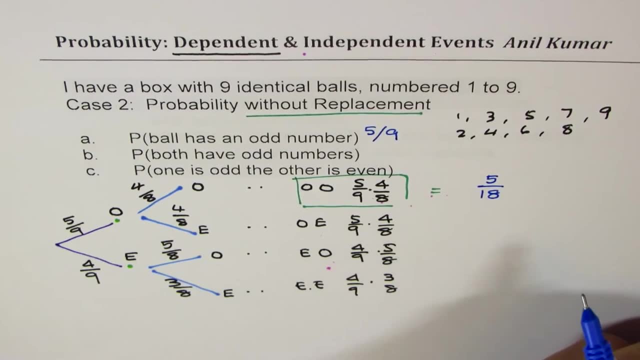 So it is. you could simplify this. it becomes half. so 5 over 18. right, in a simplified form, You can write 20 over 72 and then reduce also. Now the other case is: one is odd, the other is even. So that means we are talking about any of these two combinations. 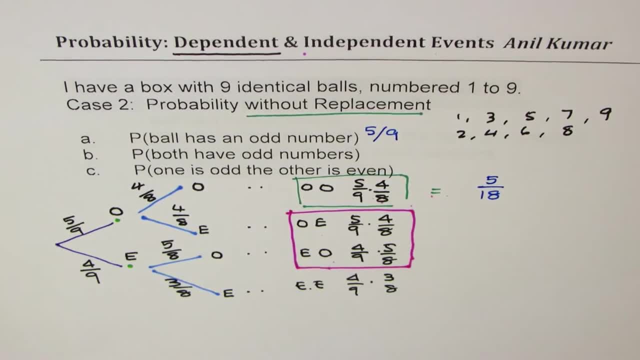 Any of these two combinations correct. So that gives you the probability. So for b is 5 over 18. let me write this down. and here the combination is 5 over 9, and I could write 4 over 8 as 1 over 2. 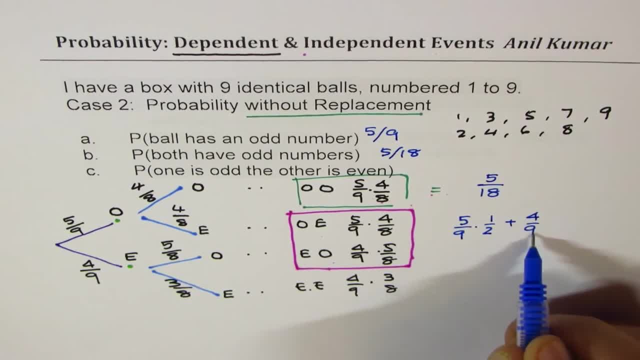 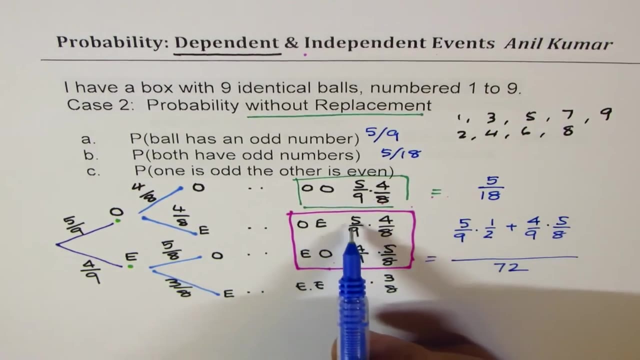 plus 4 over 9 times 5 over 8.. See as so. we will prefer to write 72, which is a common denominator, nine times 8, 72, and the numerator will be: Let me write 20 here, right, So 25 times 4 plus 20.. So that gives you 20 plus 20 as 40.. 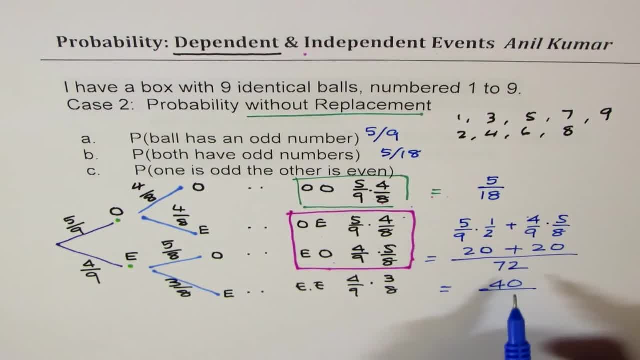 I could have simplified, right, yeah, so 40 over 72, which gives you the result. you can simplify. you can write: divide both by 4 so you get 10 over divide by 4, 4 times 1 and 32 is 18, and that could. 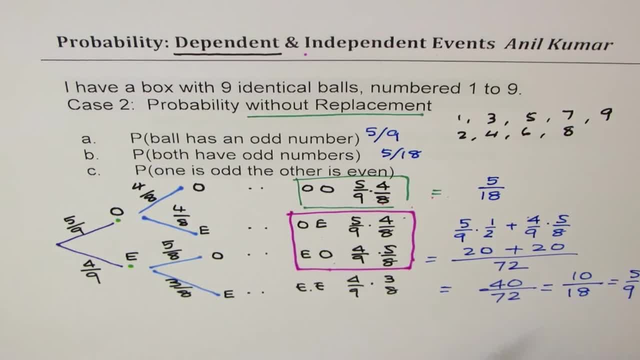 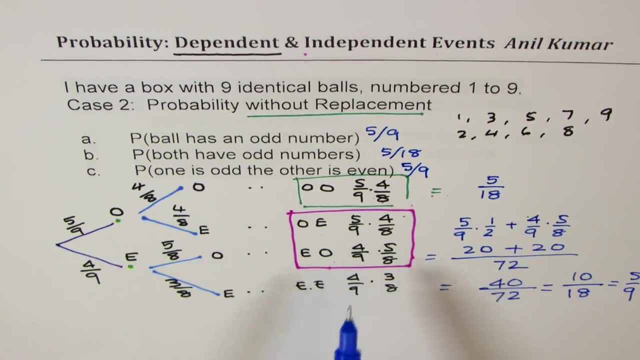 be written as you could further divide by 2, get 5 over 9 as your result, right? so we get an answer here: 5 over 9, as without replacement, one is odd, the other is even right. okay, you could actually do this part much simpler, as we could modify this. right, we could write this as 1 over 2, correct? 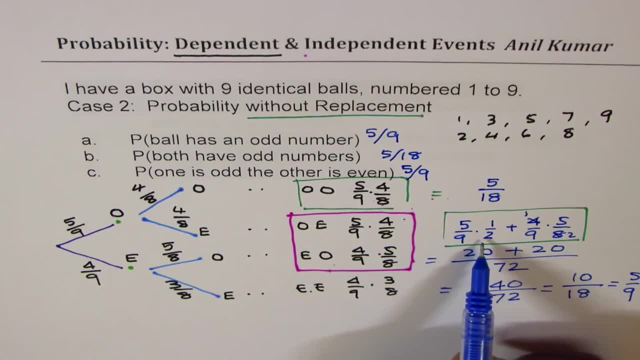 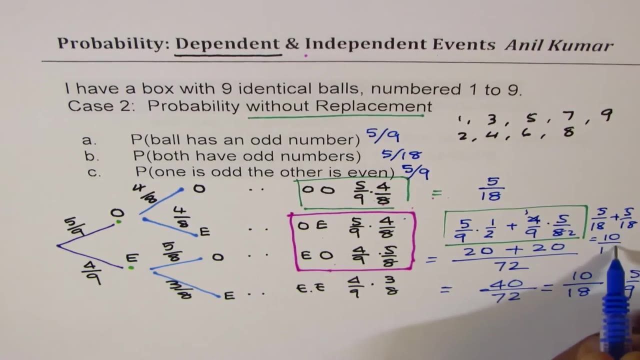 modify this and you could also write this as 5 over 18, over 5 over 18, and get the same result right as let's redo it. so it is 5 over 18 plus 5 over 18. that gives you 10 over 18, or dividing by 2. 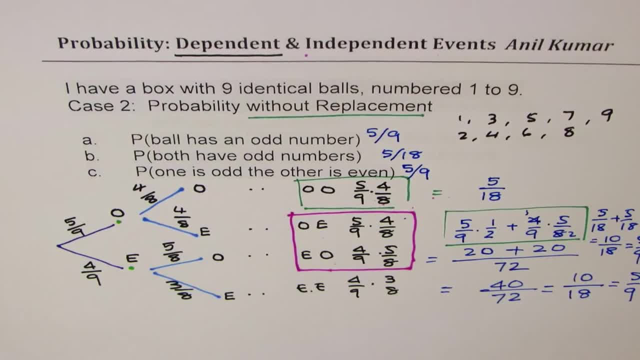 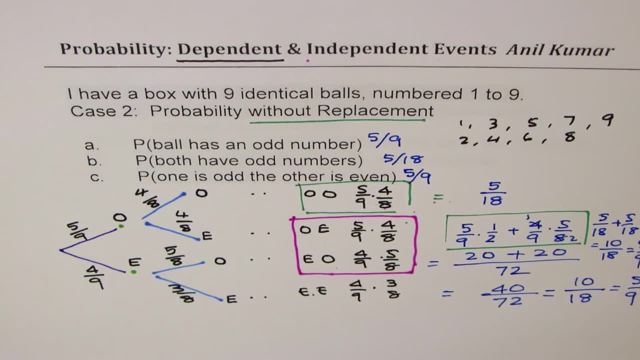 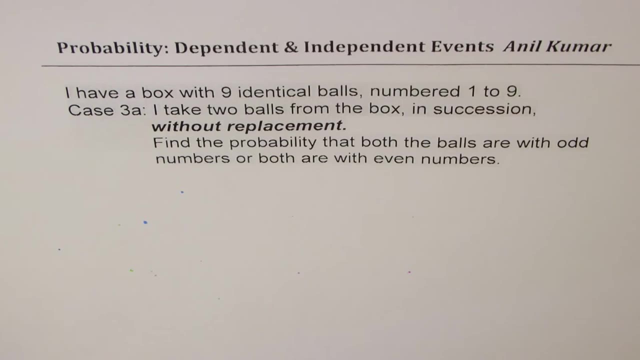 we get 5 over 9, right, so the same result. so that is how you can find the probability of the event with without replacement. okay, now let's take up the next example, where I have a box with nine identical balls numbered 1, 2, 9, case 3a. so I've actually modified this. 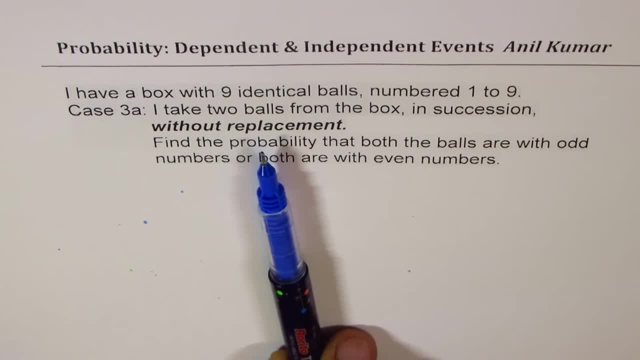 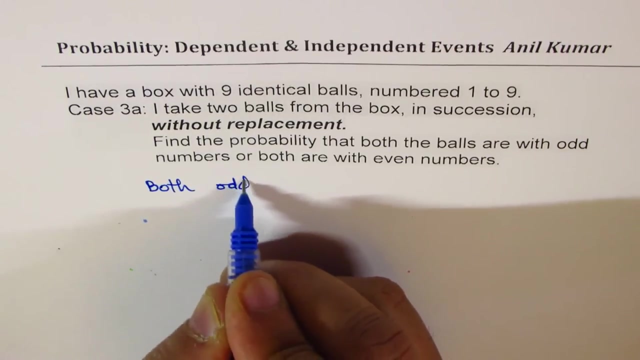 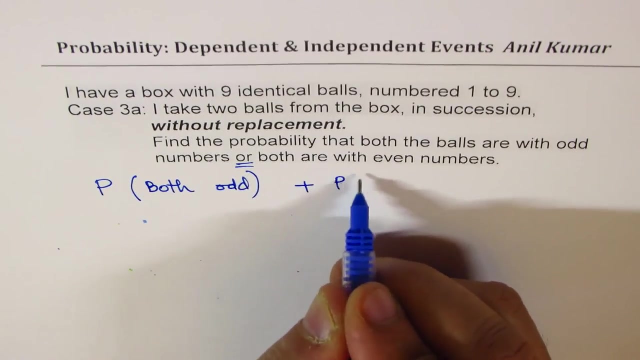 question a bit. we'll do without replacement. and with replacement I take two balls from the box in succession, one after the other, without replacement. find the probability that both the balls are with odd numbers or both are with even numbers. so we are saying or so that probability. when we say or, that means we have to add the second probability. 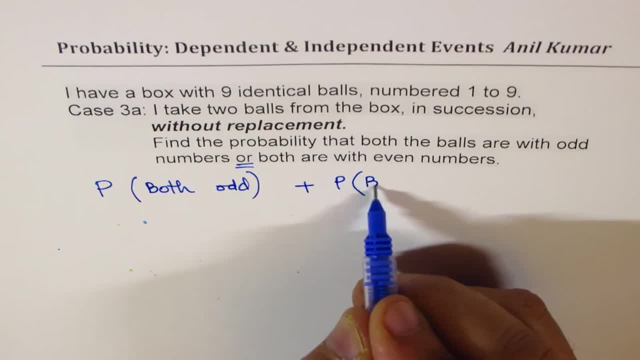 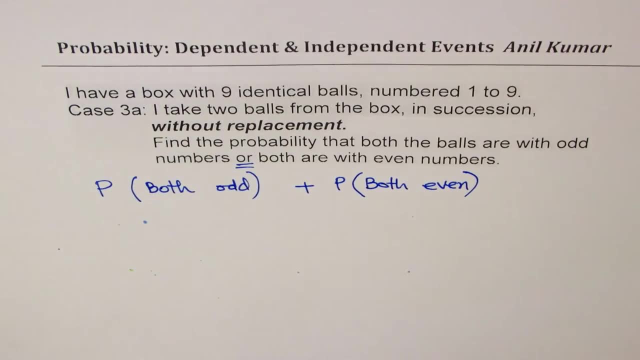 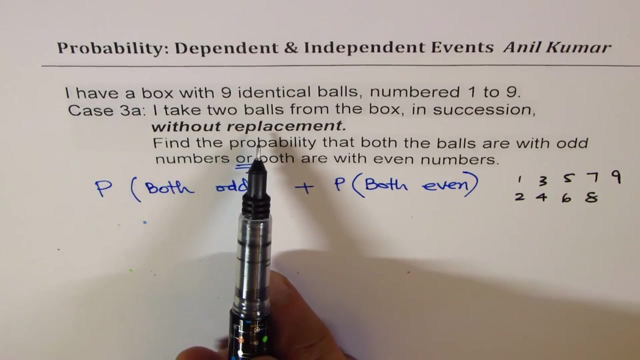 when both are evens, right. so both even. and this is the case of without replacement. so we are working with the same numbers, which are 1, 2, 3, 4, 5, 6, 7, 8 and 9. so both odd, without replacement. without replacement means it is: 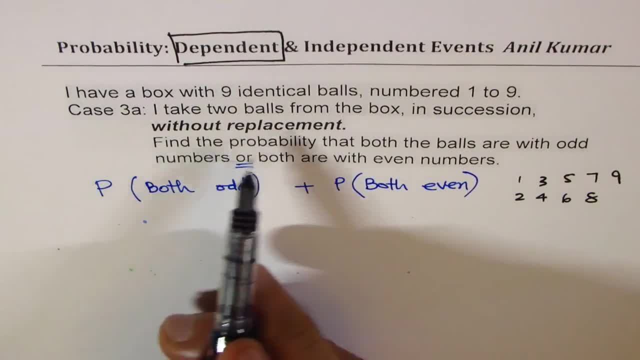 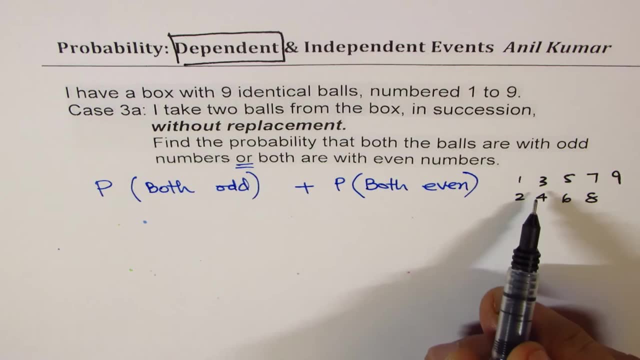 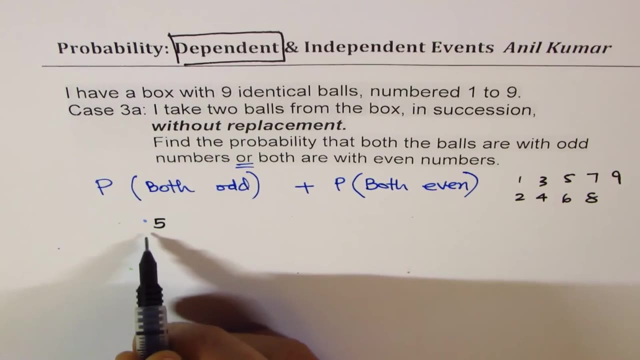 dependent event. right, so it is a dependent event without replacement. the number reduces, correct. so first time if i pick up a odd number, my probability is, since there are 1, 2, 3, 4, 5 odd numbers, so 1, 2 time it is 5 over total of 9. once odd number has been picked, one less and the 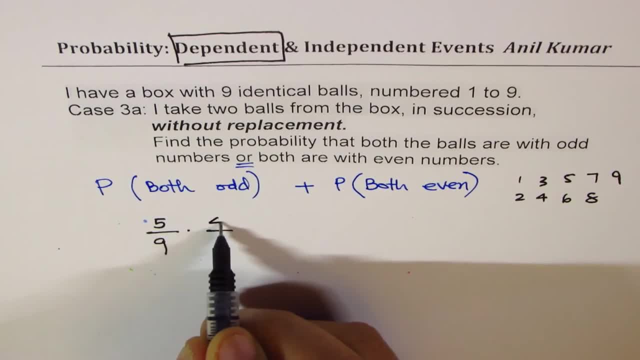 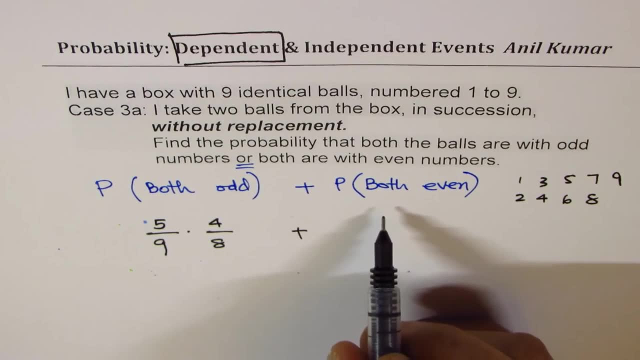 number of all also reduces, as we saw earlier. so it is 4 over 8. next odd. is it okay- and here we'll add to this both evens first time, if I have to pick even 4 out of 9 once even number has been picked? total numbers in our sample space. 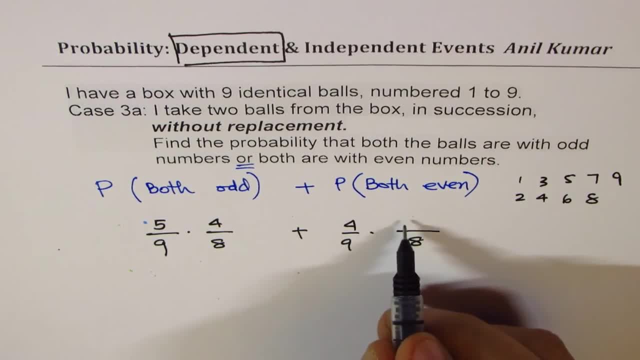 is 8, but the number of even balls have reduced to 3, so that becomes your answer. is that fine? so we can now simplify this and write this as 5 over 9 times half. plus we can divide this, we get 3: 3 over 9, can. 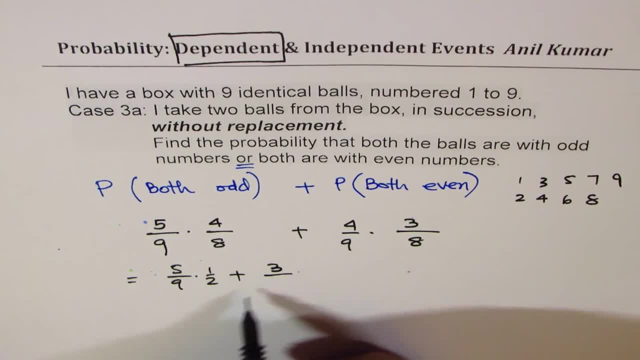 also be 5 over 9, so we can divide this. we get 3. 3 over 9 can also be 5 over 9. can also be simplified as 1 over 3, but I'll keep it same, since the denominators 18 is easy to add right. so 3 over 9 times half, 3 over 9 times half, so we get 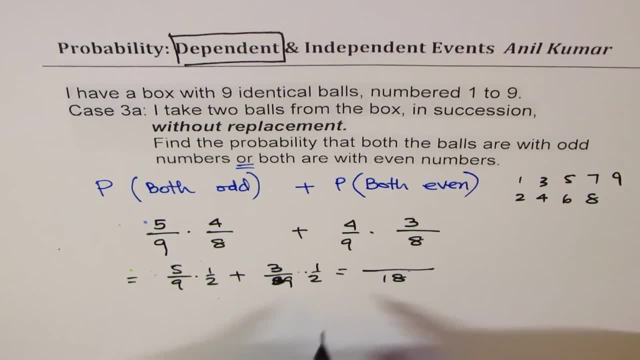 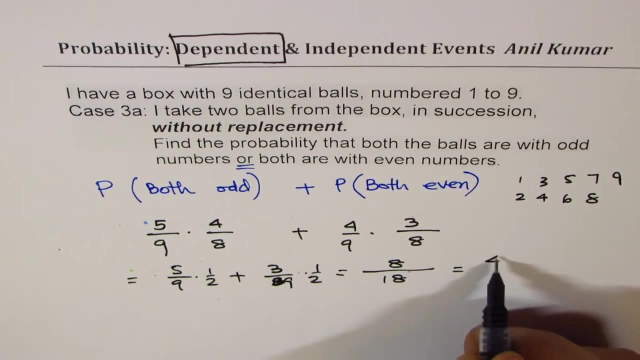 this is 9. okay, so the denominator common is 18, the numerator is 5 plus 3, 8, which can be simplified dividing by 2, 4 over 9, right? so the probability, without replacement, of getting both odd or both even is 4 over 9. great, so that is our answer. now here is 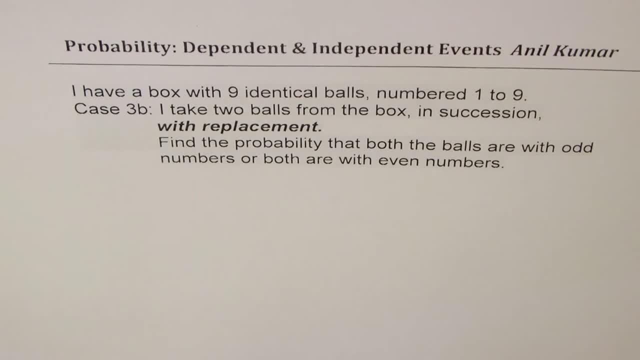 case 3b, where we'll perform the same thing with replacement right. so I have a box with 9 identical balls numbered 1, 2, 9. so the numbers are 1, 2, 3, 4, 5, 6, 7, 8 and 9. 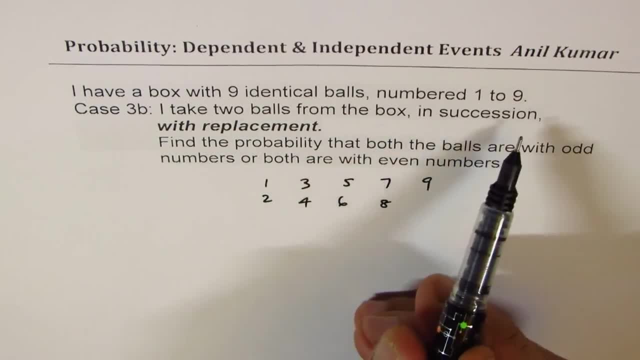 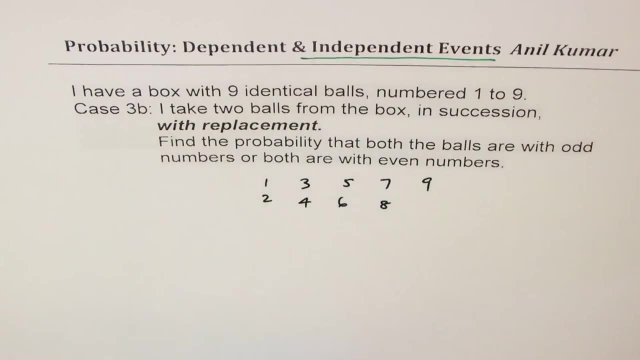 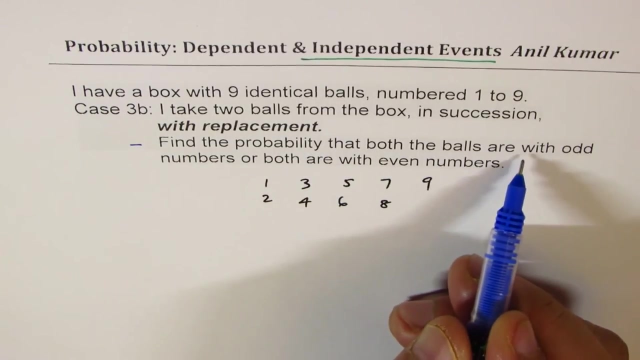 I take 2 balls from the box in succession with replacement. so that means we are not talking about independent events, right? so I think this concept is clear. it independent events. total number remains same right. probability doesn't really change. it says: find the probability that both balls are with odd numbers. we need both odd. 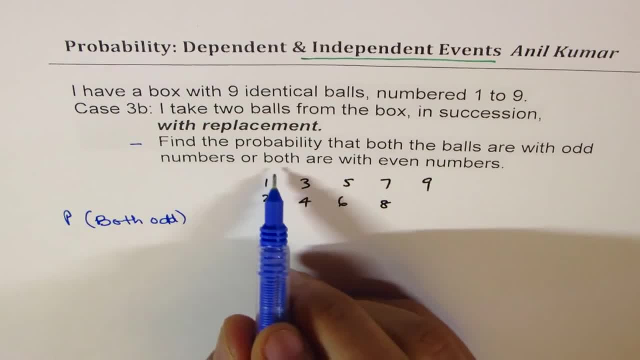 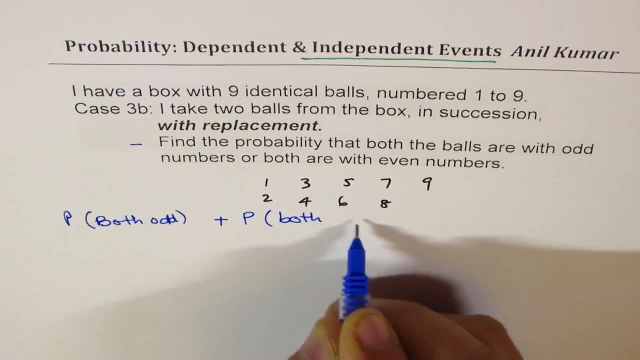 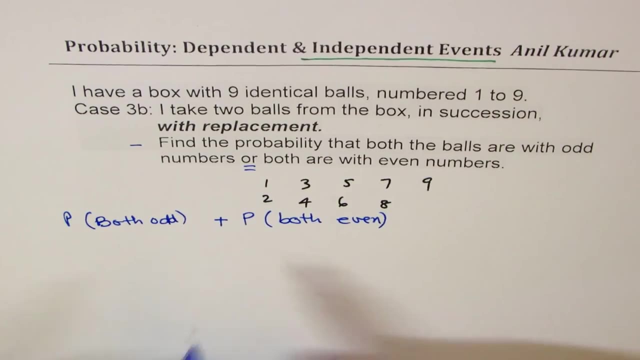 numbers plus both with even numbers, right, both even numbers. so whenever it is, or it gets added up, right, so both are. there are five out of nine. they have been replaced. it remains the same next time. so it's again 5 out of 9, which is equal to 2 over 9 times. 8 plus 2 over 9 plus 2 over 9 times 8 plus 2 over 9 times 2 over 9 times 8 plus 2 over 9 times 8 times 2 over 9 times 8 plus 2 over 9 times 8 plus 2 over 9 times 8 plus 2 over. 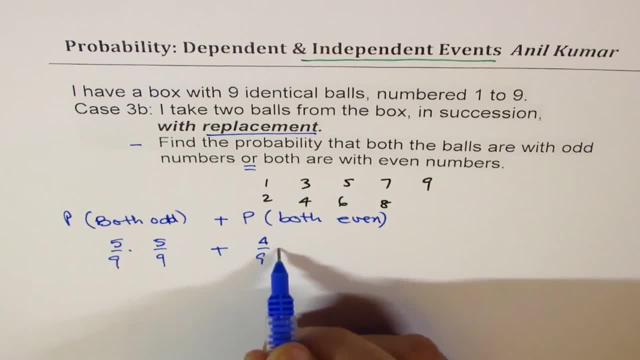 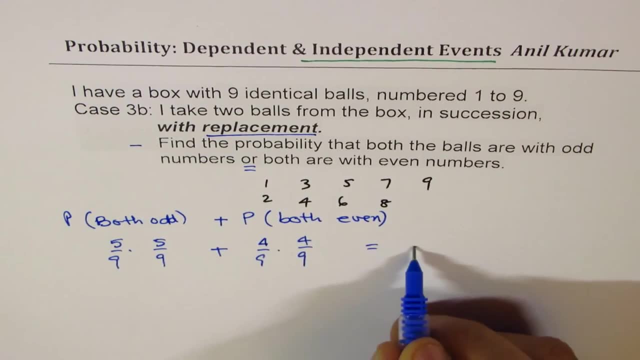 9, for even it is 4 out of 9, and again replace, so get 4 out of 9, so you can get the total as their sum is equal to 9 times 9 as 81, 25 plus 20, right, so we get the answer as 45 over 81, so that